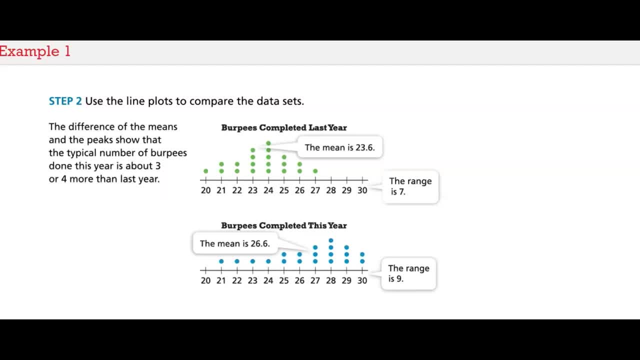 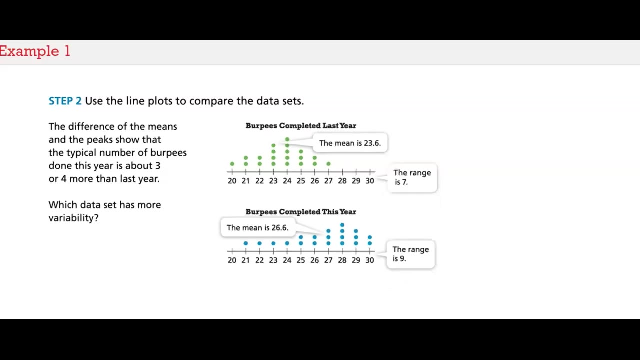 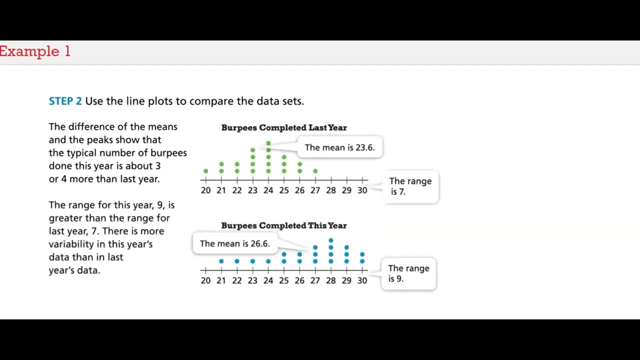 The range is 9.. The difference of the means and the peaks show that the typical number of burpees done this year is about 3 or 4 more than last year. Which dataset has more variability? Select your answer. The range for this year- 9, is greater than the range for last year, 7.. 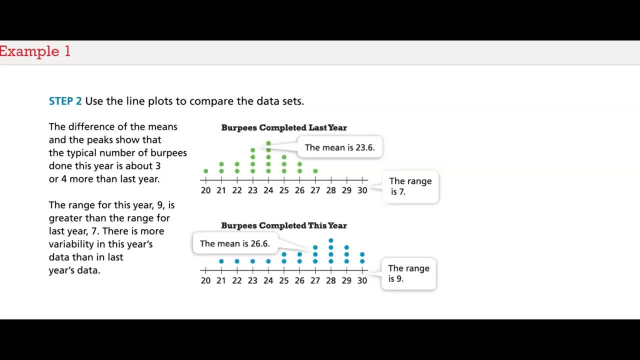 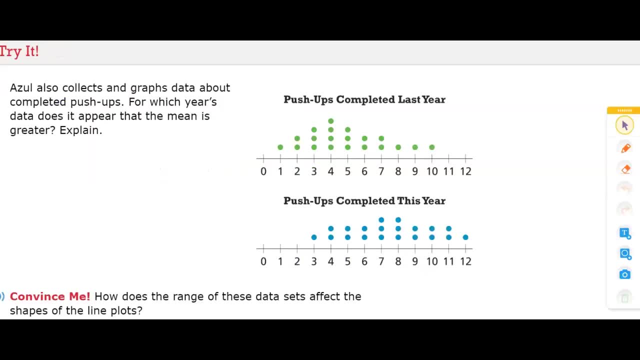 There is more variability in this year's data than in last year's data. Asul also collects and graphs data about completed pushups. For which year's data does it appear that the mean is greater? Explain: It seems that the mean is greater for this year? 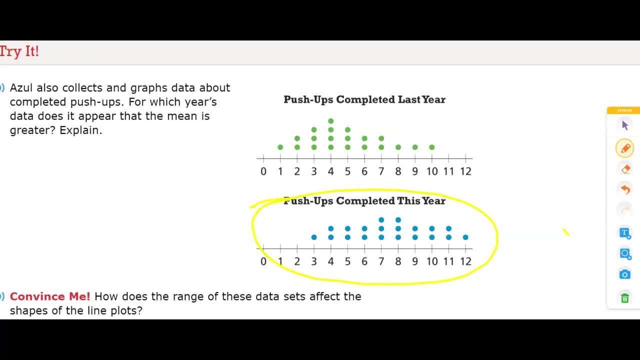 because if you look at the line plots from last year to this year, last year started at 1 and they go to 10.. The majority of the points are right here: 3,, 4, and 5.. 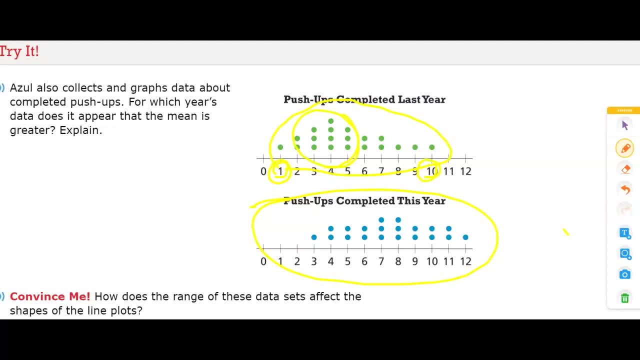 Right. And then this year, the point of the points, the dots data starts at 3 and there is some data at 12.. And the majority of the numbers of completed pushups are 7 and 8.. So just based on that identity, you see. 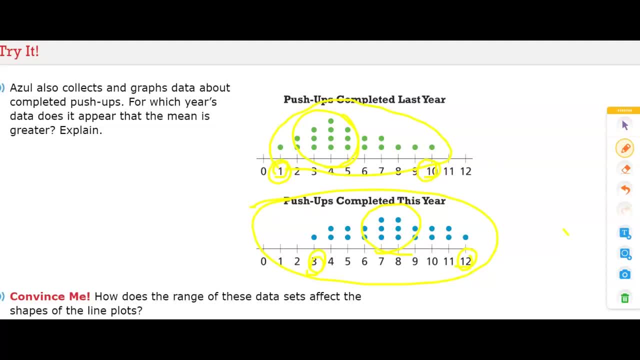 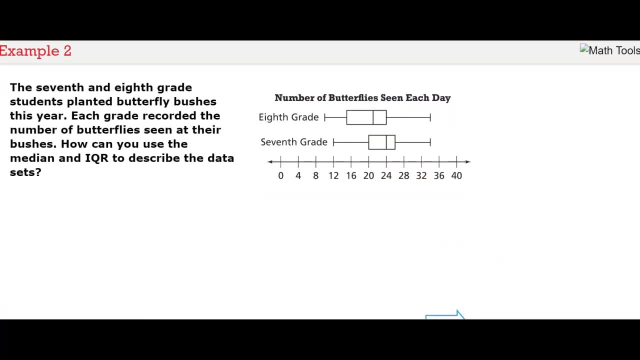 that this year's data would appear to be greater. The 7th and 8th grade students planted butterfly bushes. this year, Each grade recorded the number of butterflies seen at their bushes. How can you use the median and IQR to describe the datasets? 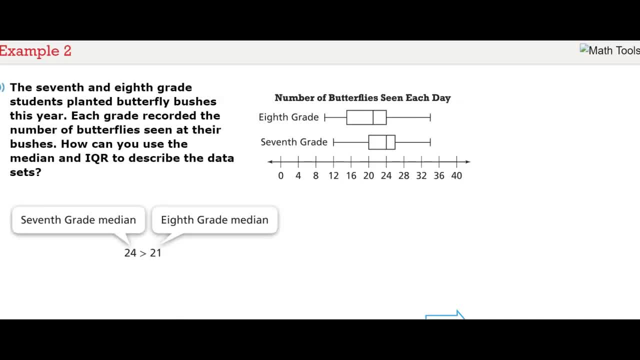 7th grade median is 24.. You notice that from here, 8th grade median is 21.. That is about here. So 24 is greater than 21.. The 8th grade IQR is 9.. Here is the IQR. 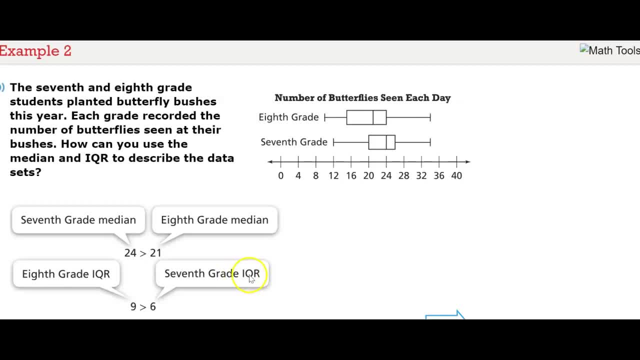 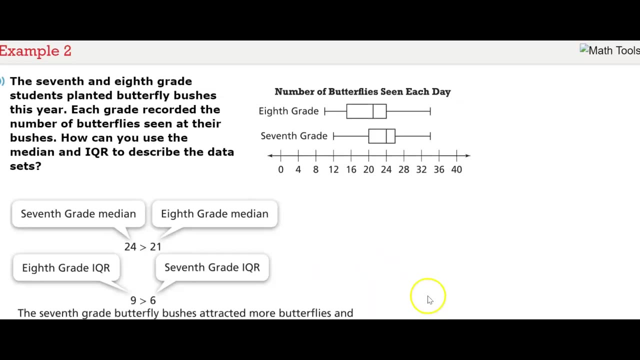 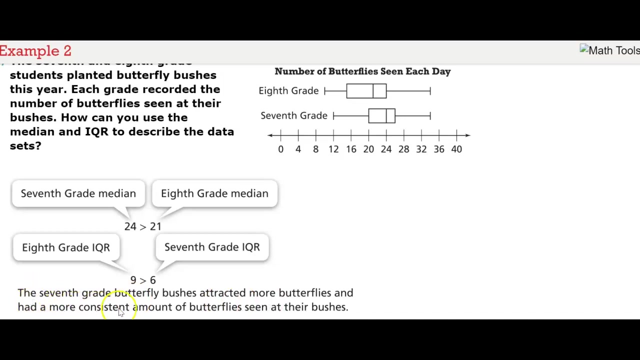 And then you have the 7th grade IQR at 6. And then 9 is greater than the 6. The 7th grade butterfly bushes attracted more butterflies and had a more consistent amount of butterflies seen at their bushes. 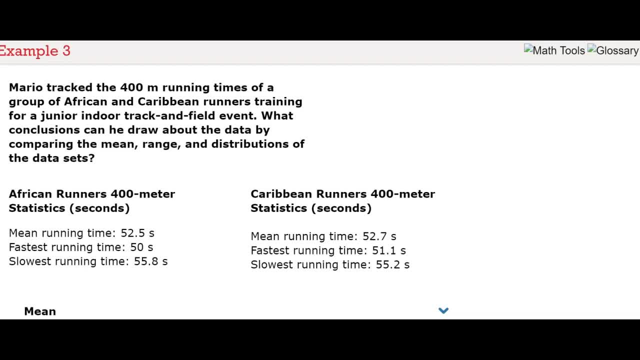 Mario tracked the 400 meters running times of a group of African and Caribbean runners training for a junior indoor track and field event. What conclusions can he draw about the data by comparing the mean range and distributions of the datasets? 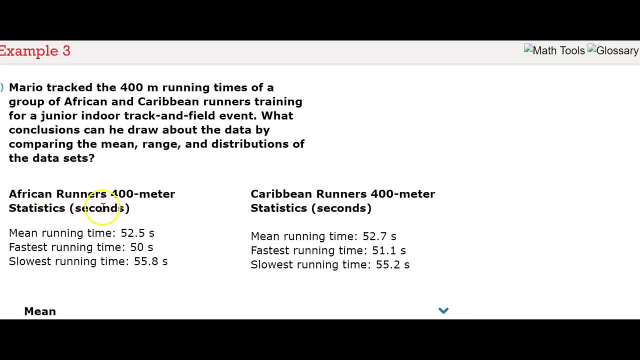 African runners' 400 meter statistics. in seconds mean running time: 52 and 5 tenths seconds. Fastest running time: 50 seconds. Slowest running time: 55 and 8 tenths seconds. Then you have the Caribbean runners' 400 meter statistics. 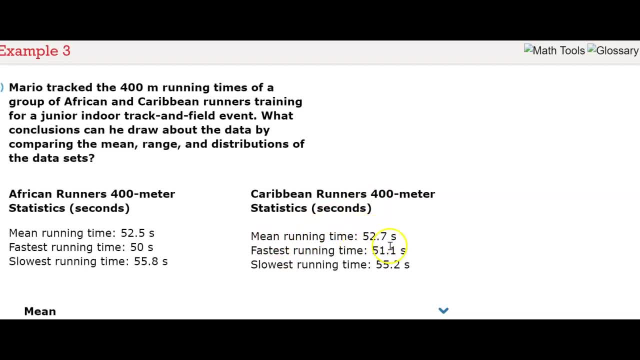 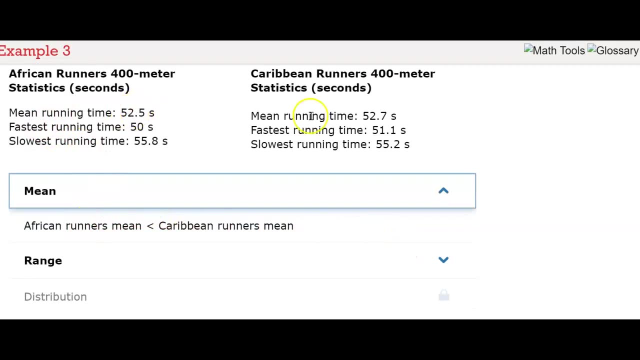 The mean running time is 52 and 7 tenths seconds. Fastest running time is 51 and 1 tenths seconds. Slowest running time is 55 and 2 tenths seconds. And then you have your mean, The African runners' mean, here. 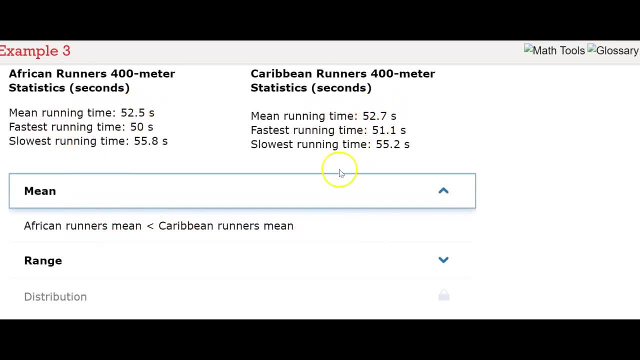 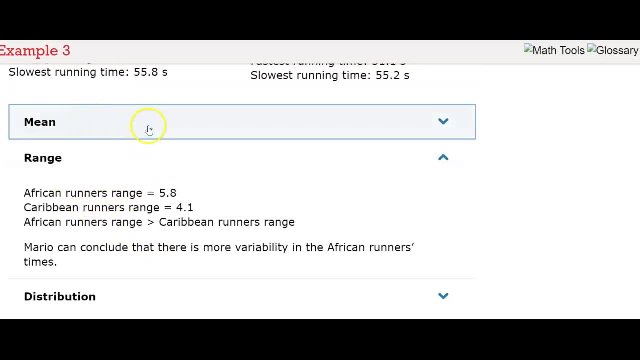 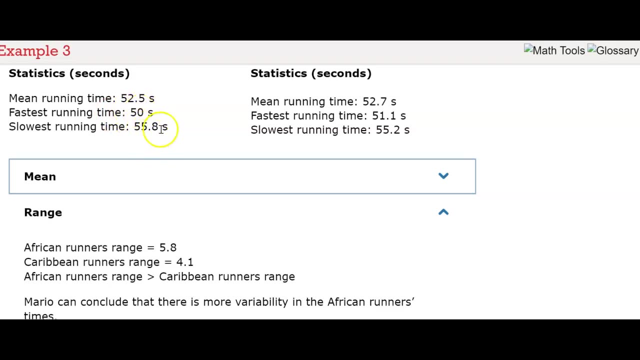 is less than the Caribbean runners' mean. Then you have your range. The African runners' range would be their fastest time subtracting their slowest time, And their range is 4 and 1 tenths for- I'm sorry- 5 and 8 tenths for the African runners. 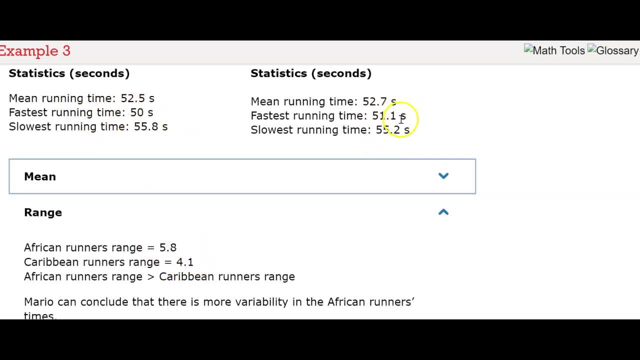 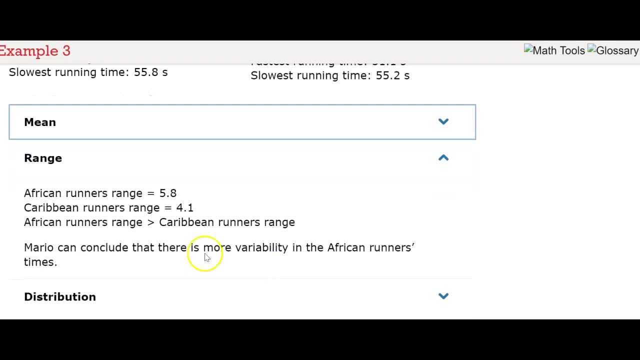 And 4 and 1 tenths for the Caribbean runners, And so the African runners' range is greater than the Caribbean runners' range. So Mario can conclude that there is more variability in the African runners' time than the Caribbean runners' time. 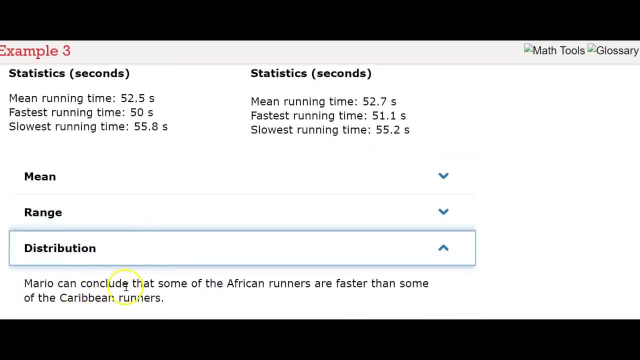 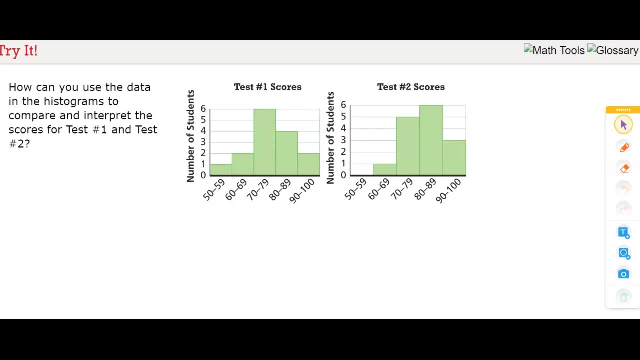 Then you look at the distribution, Mario can conclude that some of the African runners are faster than some of the Caribbean runners. How can you use the data in the histograms to compare and interpret the scores for test number 1 and test number 2??